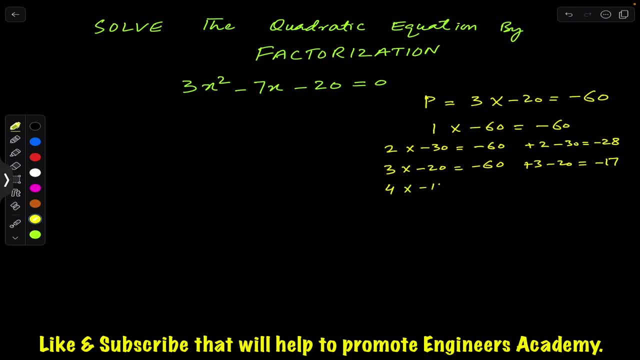 4 into minus 15 will also give us minus 60, but plus 4 minus 15.. 4 plus minus 15 is the sum of both of these numbers is again minus 11.. 5 into we can write 5 into minus 12. this is equal. this is: 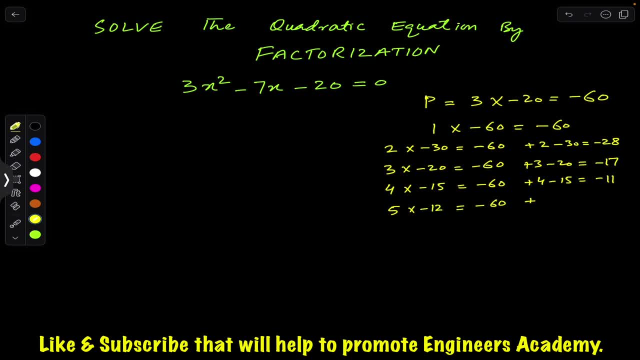 also equals to minus 60 and plus 5. this is plus 5. so plus 5 plus minus 12, this gives us minus 7.. So we got that minus 7 if we multiply 5 with minus 12.. So 5 into minus 12 is in minus 60. we got that. 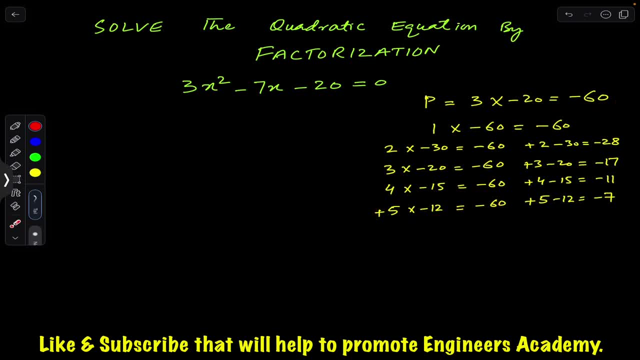 same product and the sum of both of these numbers is minus 7.. So these are the desired two numbers that we need to find right. So the method is that we need to multiply 3 with minus 20, we will get. we get some product and that product is minus 60. then we have to find such two numbers whose? 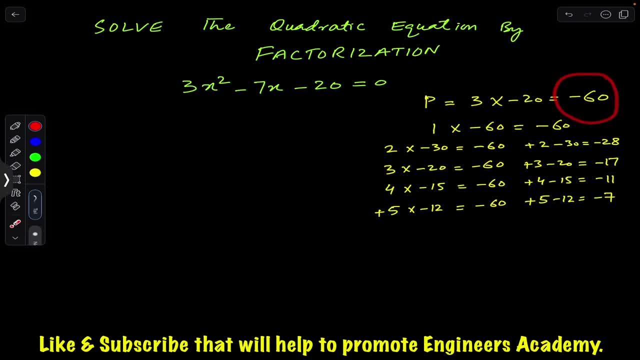 product is minus 60 and whose sum is minus 7.. So 5 and minus 12 are those two numbers whose product is minus 60 and whose sum is minus 7.. So then we can split this: minus 7, x is 5 plus 5, x minus 12, x. 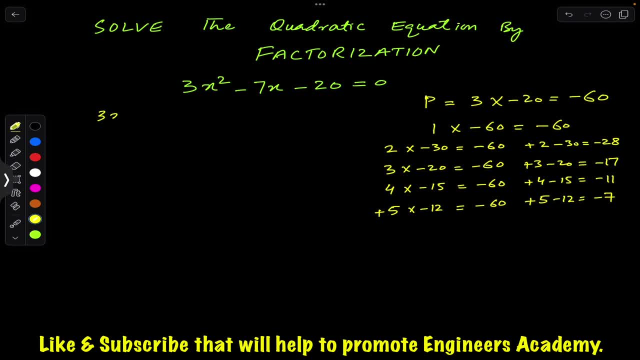 So we can write this quadratic equation like this: 3 x square. we will split this minus 7 x term into two terms and we can write this: minus 7 x is plus 5 x minus 12 x minus 20 equals to zero. So 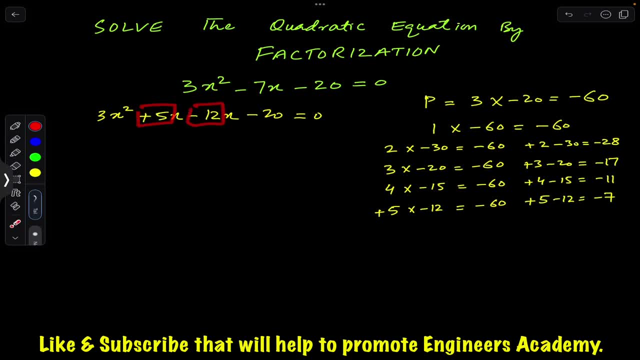 plus 5 x and minus 12 x. these are those two numbers, which gives us the sum minus 7.. So we split this term into two and if we add these two terms, we will get that same minus 7 x. So we did nothing, we only converted this minus 7 x term into two different terms and by adding these two terms, 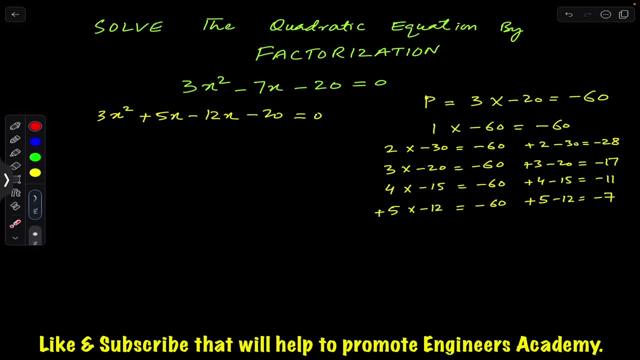 we. we are getting that same minus 7 x term. So this is 3 x square plus 5 x, minus 12, x minus 20, and now from these two terms we can take x as a common, So we can write that this will be x. 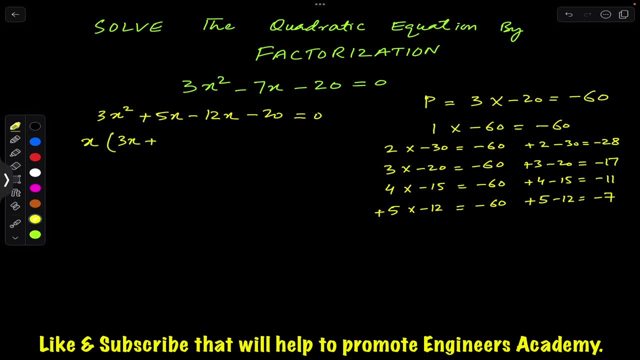 then we can write that this will be 3 x plus 5, and similarly, from both of these two terms we can get minus 4 as common. So we will write minus 4, so this will be 3 x and plus 5, and similarly. now this: 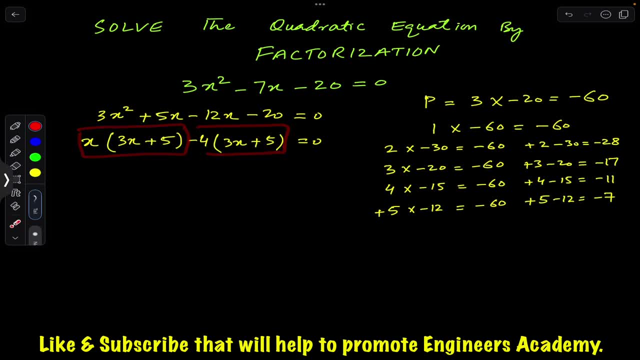 one term, and this is second term. now, from both of these terms we can take 3 x plus 5 as common. So we can write that 3 x plus 5 and we are left with x minus 4 equals to 0.. Now, now either this term: 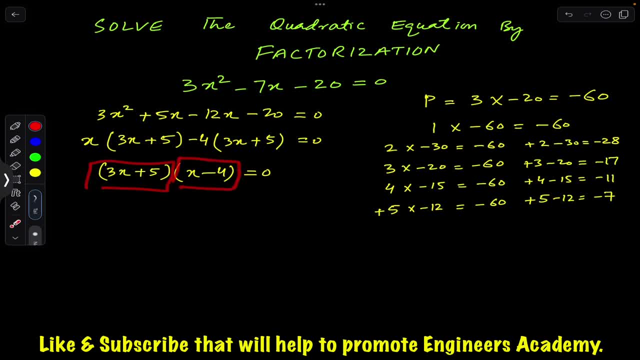 be equals to 0 now, or we can say x minus 4 is equal to 0. So we can say that 3 x plus 5 equals to 0, or x minus 4 equals to 0, or both can be equals to 0. 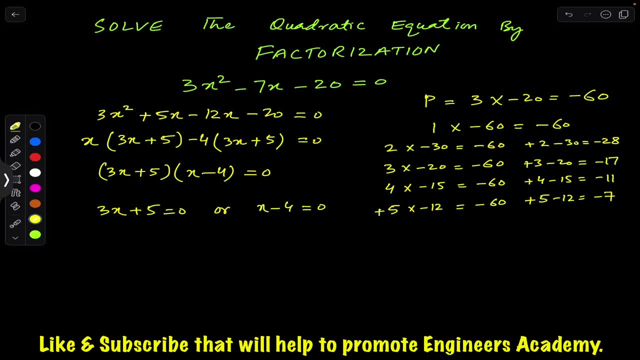 The product is 0, right? So now from this we can say that x is equal to minus 5 divided by 3, or we can say x equals to 4.. Now the solution set is: the solution set is minus 5 divided by 3, equal comma 4.. So this is the solution of this quadratic equation. 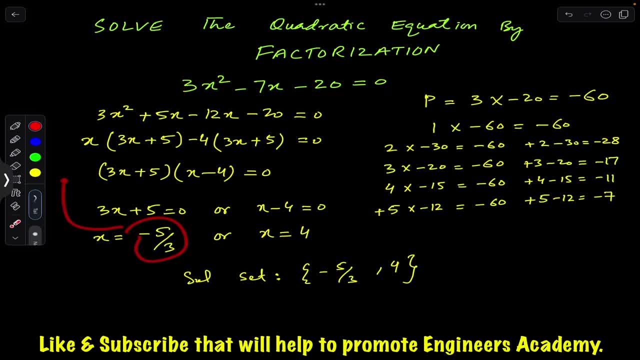 If we substitute this value of x into this value, this equation, we will get 0. and if we substitute x equals to 4 in this quadratic equation, this will be: we will get 0. so this is how we can solve the quadratic equation: by using the factorization method. let's say we have a. 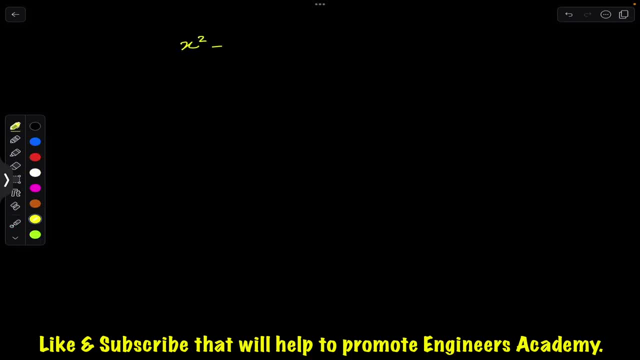 quadratic function x, square. minus x minus 20 equals to 0. so we will find the product. so the product will be this: 1 multiply by minus 20. so 1 into minus 20, we get the product equals to minus 20. now we need to find such two numbers. 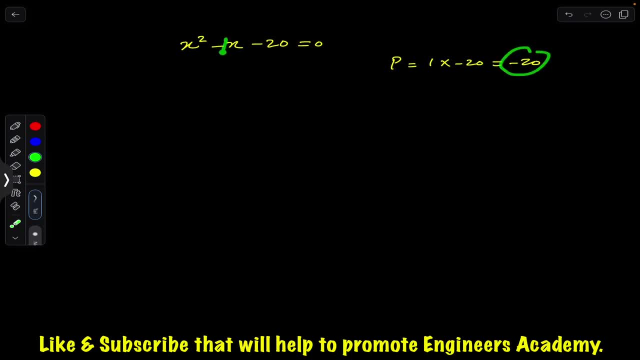 whose product is minus 20 and whose sum is minus one. so the required sum is minus 1. so 1 into minus 20. now let's say, 2 into minus 10 is again 20, but the sum is 2 plus minus 10. again the sum is not equal to minus 1. this is minus 8.